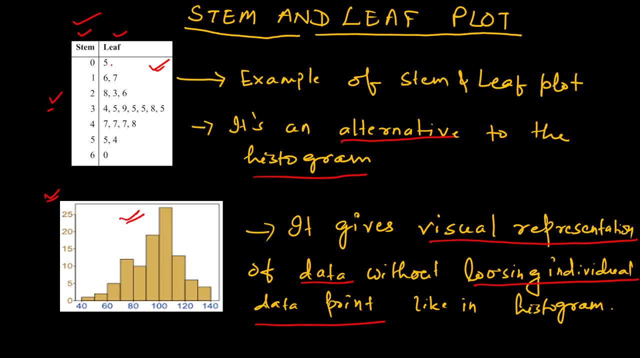 we do not lose the individual data points, Like in this case. the individual data points are represented on the plot. So this particular, you know, this particular number is nothing but 5 and this particular number and nothing but 16 and 17.. 16 and 17.. So, if I would like, if I would make it into a series of numbers, the numbers would be 5 and then 16 and then 17.. So, if I would like, if I would make it into a series of numbers, the numbers would be 5 and then 16 and then 17.. So, if I would like, if I would make it into a series of numbers, the numbers would be 5 and then 16 and then 17.. So, if I would like, if I would make it into a series of numbers, the numbers would be 5 and then 16 and then 17.. So, if I would like, if I would make it into a series of numbers, the numbers would be 5 and then 16 and then 17.. So, if I would like, if I would make it into a series of numbers, the numbers would be 5 and 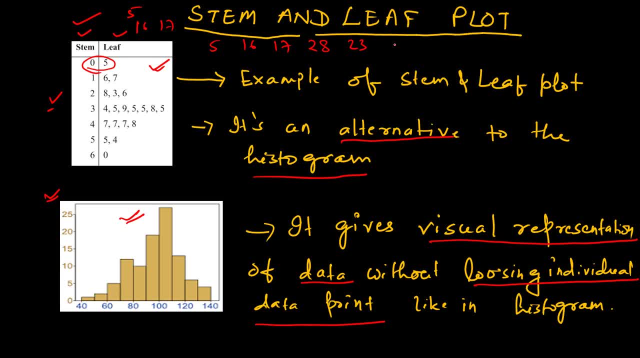 and then 28,, 23,, 26.. So that's the way we can, you know, get back to the original number series. Now, how do we construct this series again into statement leaf? We'll just learn in the next slide. So the idea is that it doesn't lose the individual data point which is, you know which. 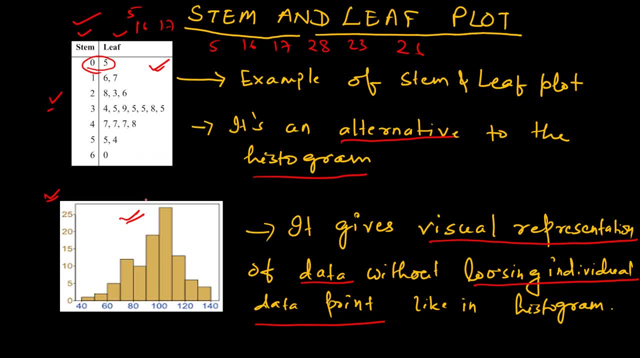 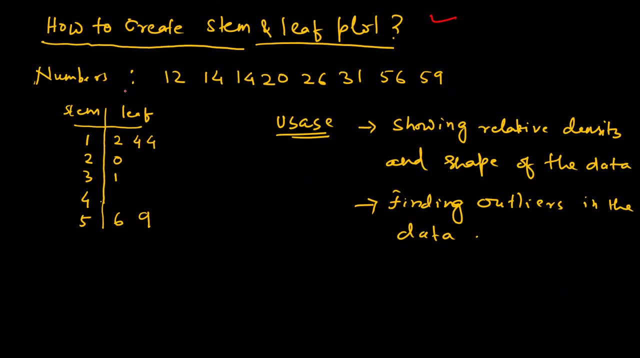 is not found on the histogram, and that's a demerit of using histograms. So how do we create this statement leaf plot? Well, let's take an example here. So I've got a number series and the first thing to do is that to sort it in ascending order. So the number series is from 12, 14 and 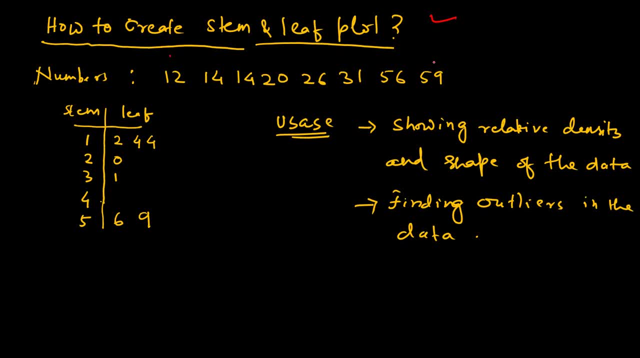 another 14,, 20,, 26,, 31,, 56 and 59. Now this series we want to represent on the statement leaf plot. So how do we do that? So first notice what is in the leftmost side of the number, or 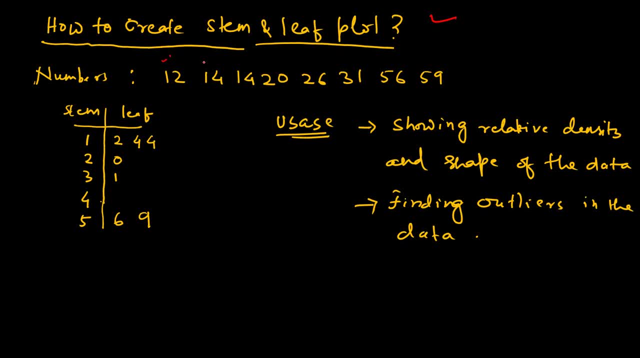 like in this case, the decimal number. It's 1. again here it's also 1, 1, 2, 2 and 3, 5 and 5.. So this is the decimal number. So what we'll do is that we'll take the extreme number or the. 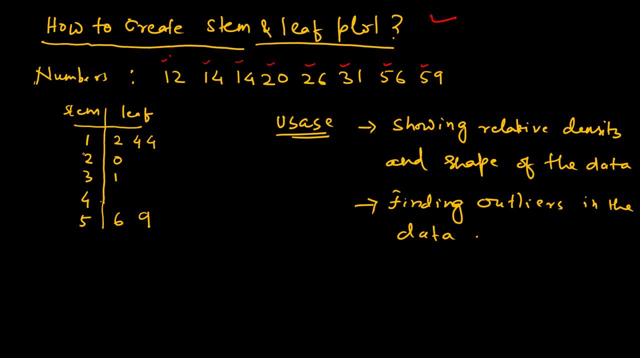 first digit of the number and we call it a statement and it starts with 1 and ends at 5.. So in between we have got. the 4 is missing, So we have 1, and then we have 2,, 3, there is no 4 and then we have 5.. So what we do is that we put these numbers 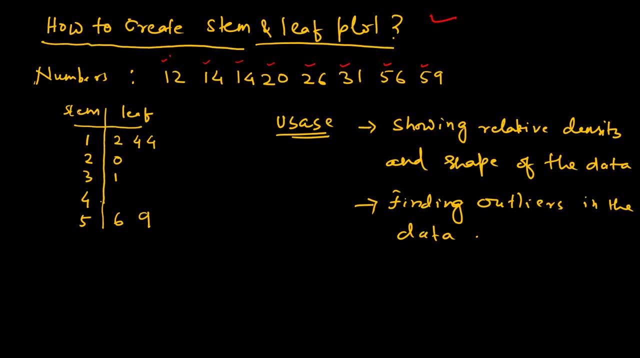 in the left side and we are calling it as tail, So we put 1,, 2,, 3,, 4 and 5.. Remember that we do not have 4, but still we need to put 4.. We cannot have a gap, So we need to put 4 over there. 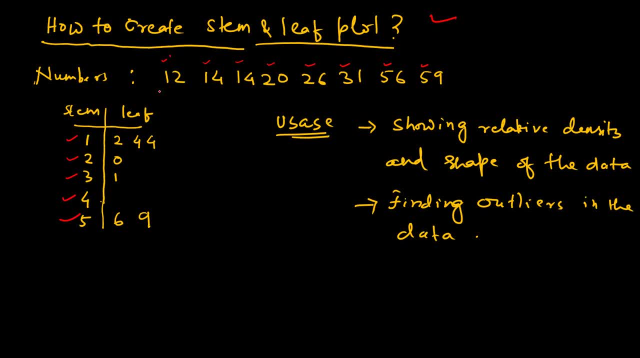 Then against 1, how many numbers are there? Well, in 12 you have got 1 and 2. Then 1,, then in the leaf portion I put 2. And then the next number is 14.. So what I do is that right next to that I put: 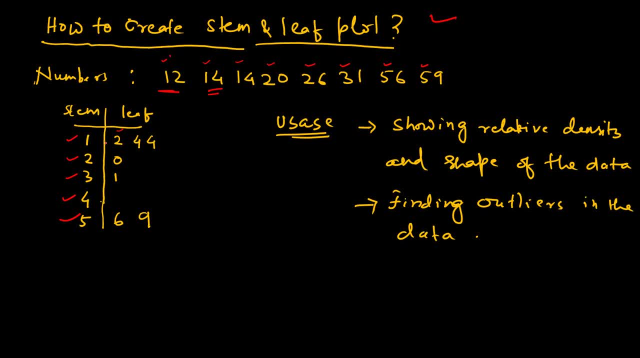 4.. So that is how we understand. So 1, 2, first number, and then 1, 4. Then we have got another 14. So that is again 1, 4. And the next one is 20. So we go to the. 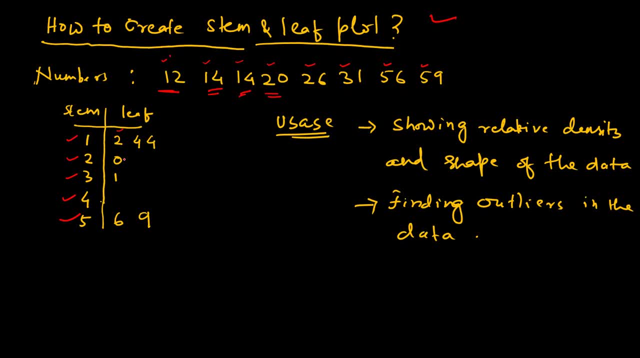 one step below and then, against 2, we got this 0. So we have 20 and there is no. you know, okay, we have another number in 20.. So that is 26.. So we will put 6 over here. Yeah, I just missed that. Okay, so we have 20 and then we have 26.. Similarly, in the 30s, we have got. 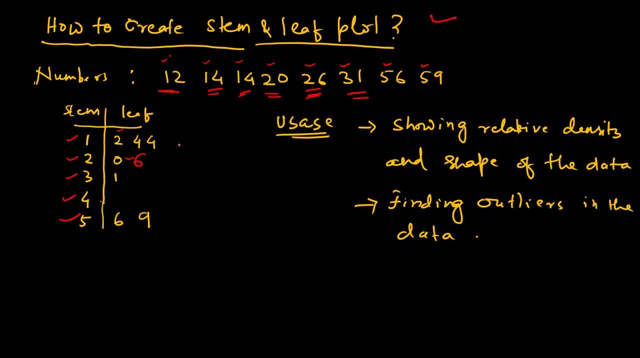 31. So against 3 we put 1, and there is no number. within you know, 20 to 30. So we go one step below and then, against 4, there is no number, So we just leave it back, And then in 50s we have got 56 and 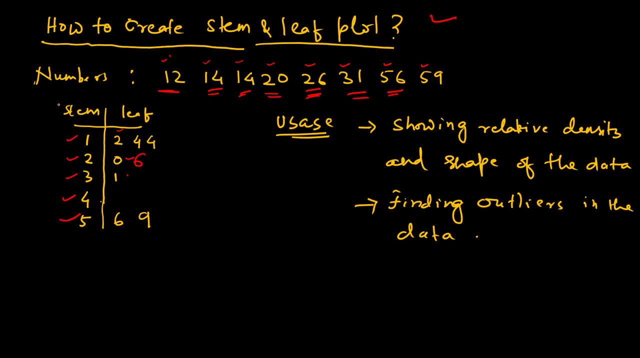 59. So we put 6 and 9.. And now this is how the leaf plot look like. So we represent the number of, or the frequency of data point in each. you know, You know, in each bean, but we do not lose the actual data points, Right? So it similar to. 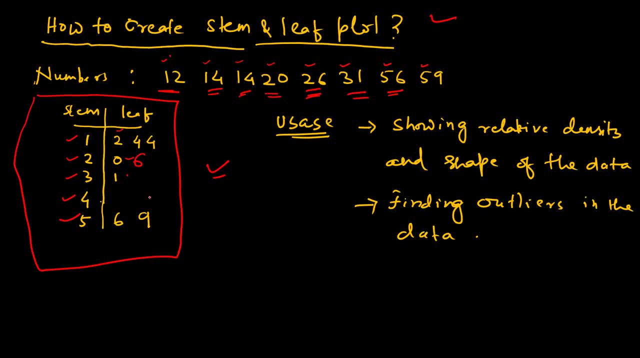 histogram, but it gives you know additional advantage that you can actually look at or get back to your actual data series from the same and leaf plot. So where is it used actually? So the first thing that is for which this is used is to show the relative density and shape of the data.